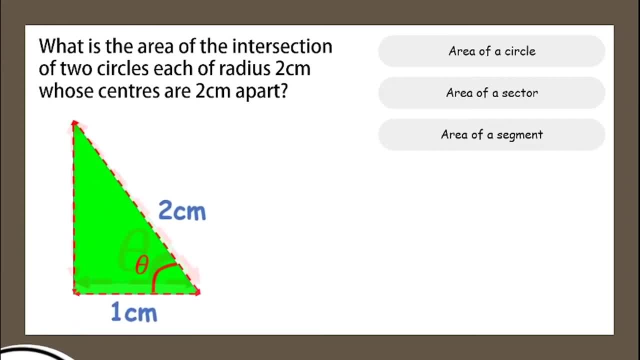 So that produces this right angled triangle And from here I can apply some trigonometry. I didn't even expect to use trigonometry. I can apply some trigonometry to try and find the angle. So theta is going to be the inverse cosine of 1 over 2, giving me 60 degrees. 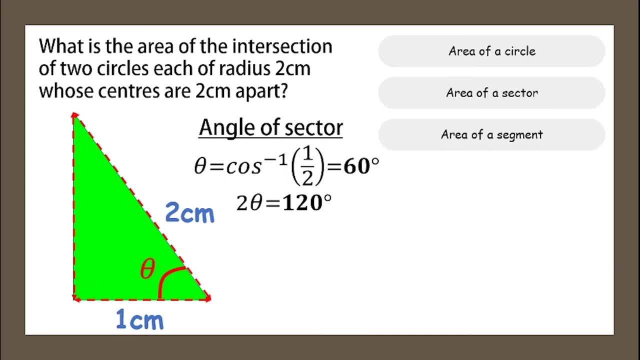 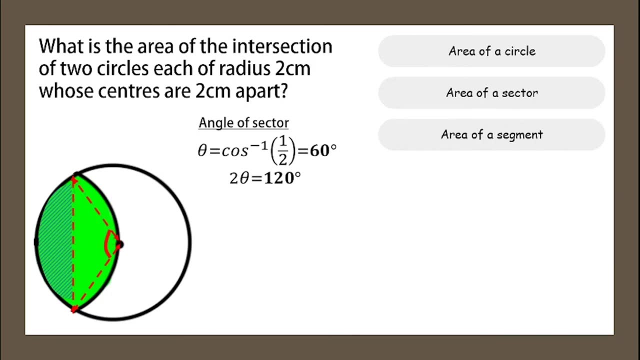 So theta here is 60 degrees, but I'm also interested in 2 theta, which would be the entire inner angle on this diagram. 2 theta equals 120 degrees. Let's go with 120 in the diagram. So what can I do from here? 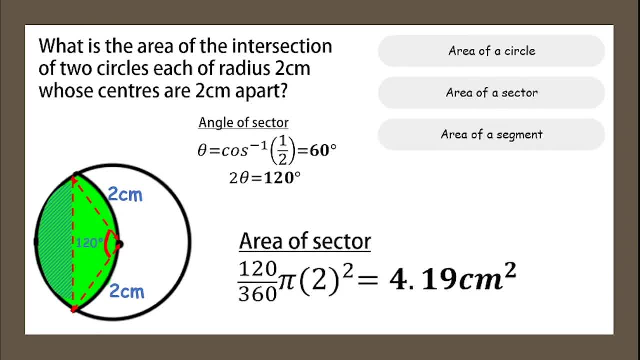 I can find the area of the sector. It's going to be a fraction of the area of the entire circle And that fraction is 120 over 360.. And if I apply that to the formula for the area of a circle, I get 4.19cm squared. 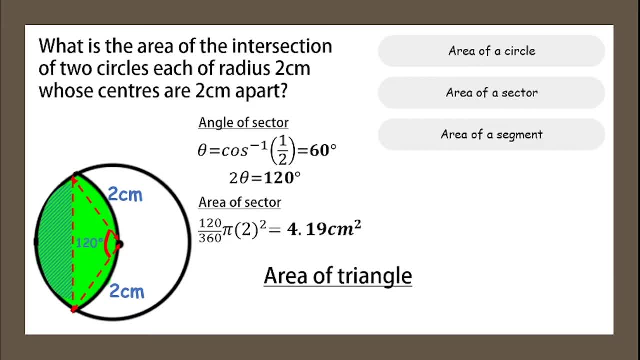 So that's the area of the sector. The sector is like a slice of cake. Let's find the area of the triangle. Well, I'm going to use half AB sine C, And in this case A and B are both 2.. 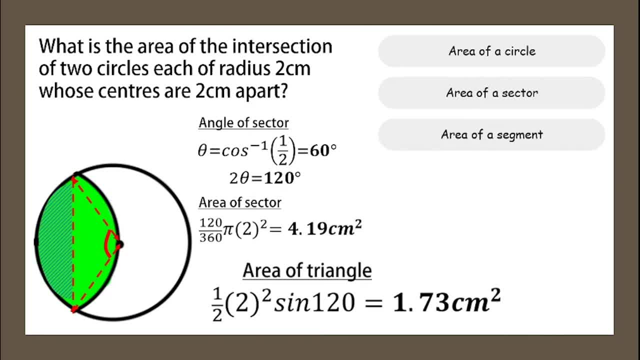 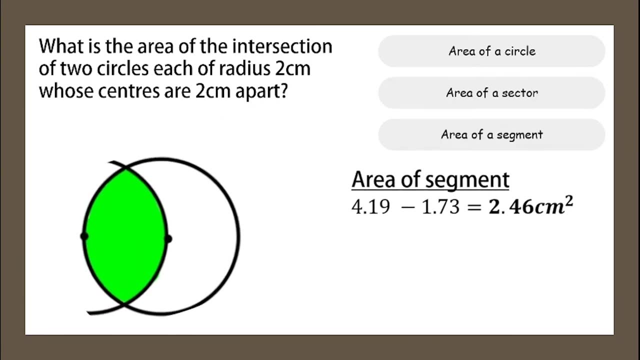 The angle is 120.. I get an area of 1.73cm squared. Okay, The segment I'm going to get from subtracting the triangle away from the sector. That leaves an area of 2.46cm squared. Alright. 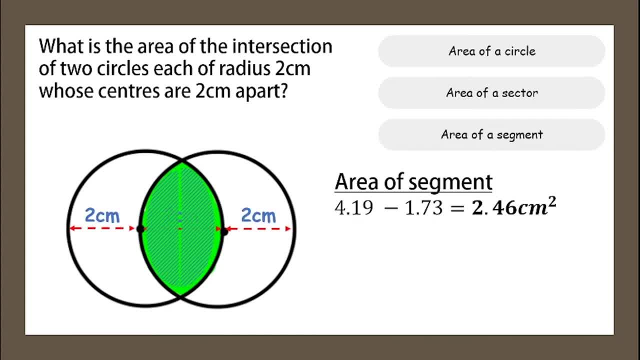 So I've got the area of the segment, as I wanted to begin with, But this shaded area looks like it's two segments. These two segments would be exactly the same. The area of the intersection is 2 multiplied by 2.46.. 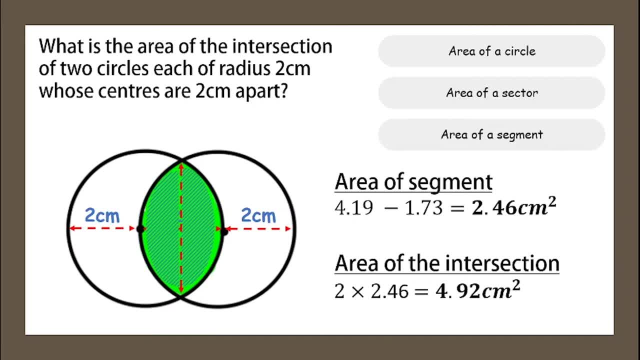 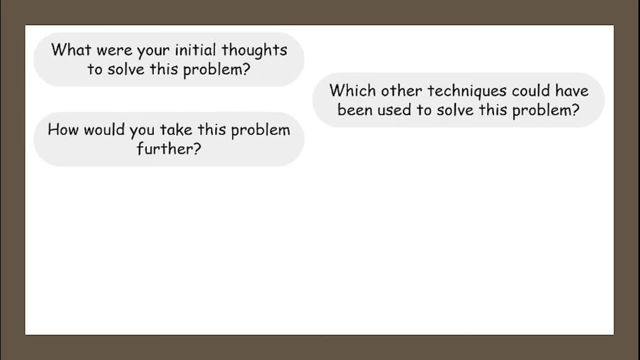 Gives me an answer of 4.92cm squared. Using a little bit of estimation to check if my answer is sensible, I know that one of these circles has an area of roughly 12cm squared. So for the segment to be roughly 2.5cm squared does seem sensible to me at the moment. So I'm happy that I've got a reasonably accurate answer. I can already think of a couple of alternate approaches to this question And, if you can just throw them in the comments so we can discuss these further, Which different mathematical techniques could have been used?